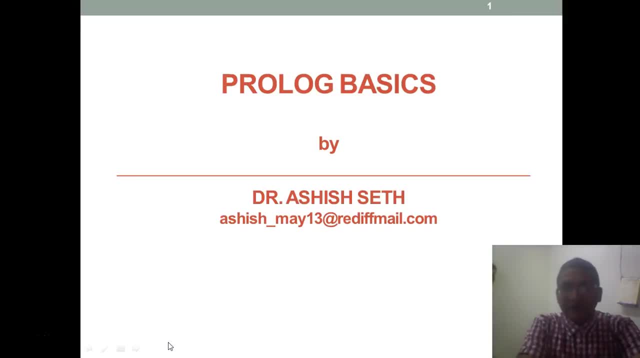 Hello friends. so in today's session we will learn about the basics of Prologue. Prologue stands for programming logic. Prologue is a programming language that uses the principle of logical reasoning to answer the queries. So basically, in Prologue, our objective is to design a knowledge. 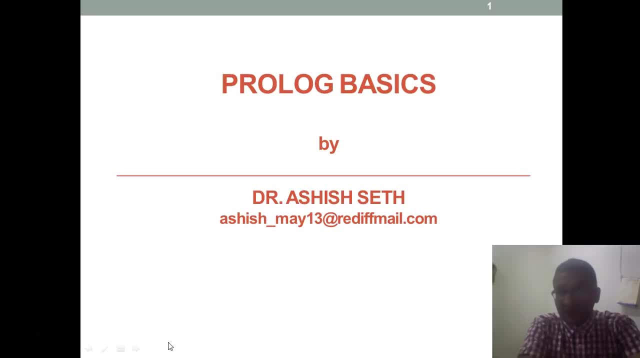 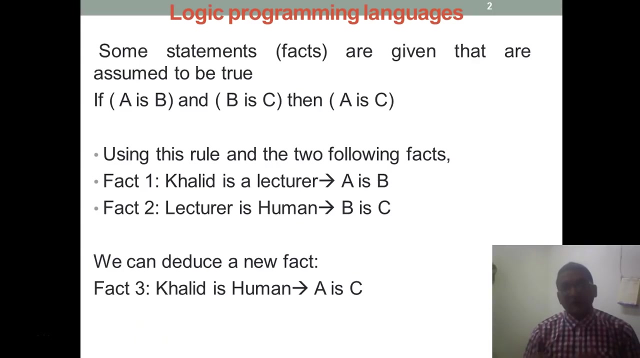 base. Knowledge base is something which contains a fact, and the rules Knowledge base has the capability to induce certain new facts out of the existing facts. So we will see So. first we will see what the fact is. So the fact is the statement which are assumed to be true. So let us take an example: If A is B, 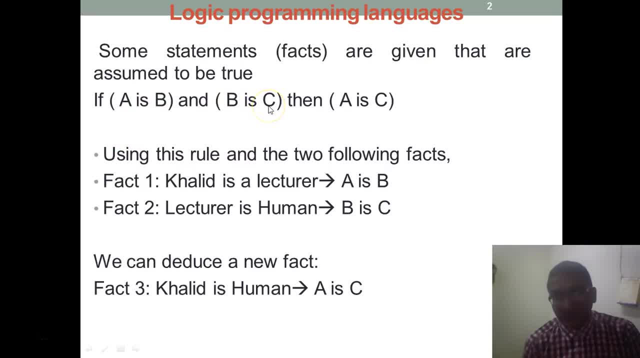 is given to us and also, if it is given that B is C, then we can induce that A is C. Similarly, if we see the other example, Let us say the two facts are given to us. Fact one says Khalid is a lecturer and we can refer this as A is B, that is, Khalid is a lecturer. The second fact: 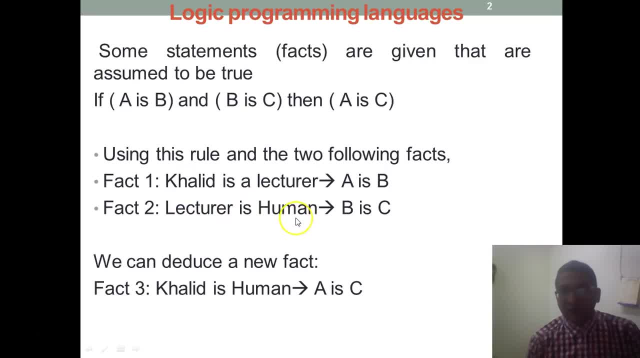 is given lecturer is human, So we can write as B is C. So if A is B and B is C, we can easily induce that A is C. That means Khalid is a human. So this is a small example, just to get the understanding. 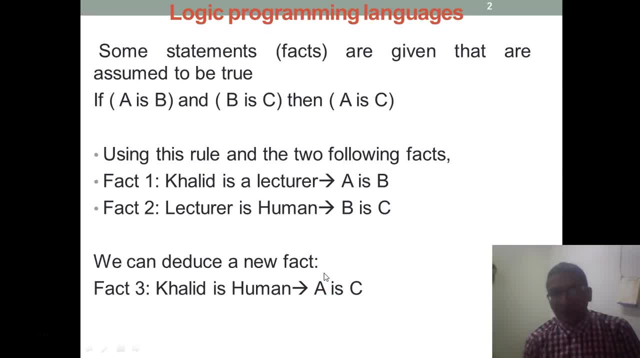 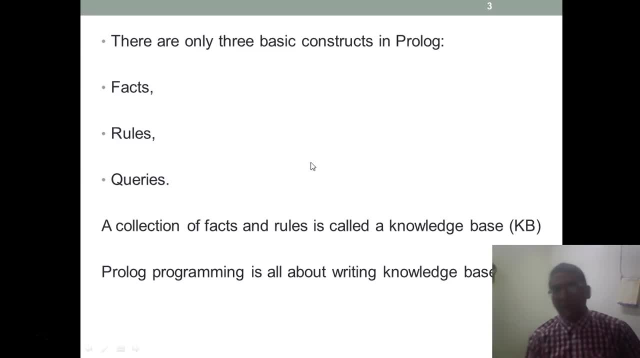 that how to induce a new facts out of the given facts. So basically, if you look in the Prologue, there are three basic constructs. One is the facts. So basically the facts are used to state the things that are unconditionally true of the domain of interest. 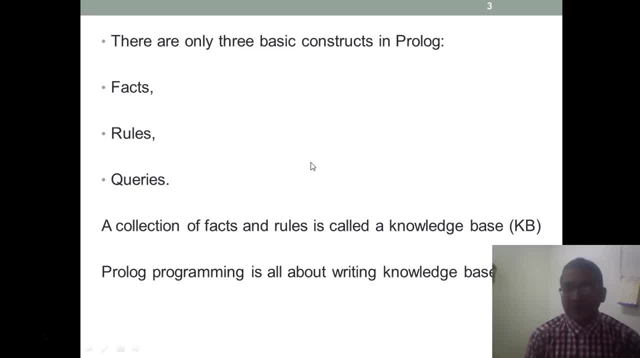 These are the statements which we assume to be true. Rules are also used to state the information that are unconditionally true of the domain of interest. So, basically, when we talk of Prologue, our objective is to create a knowledge base, and knowledge base is just a collection of facts and rules. So what we want here is that knowledge base is nothing but is a collection of facts and rules. 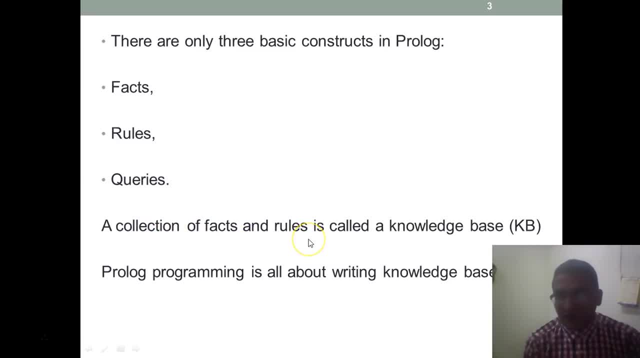 So knowledge base is just a collection of facts and rules. So when we try to make a knowledge base for an agent, we have to identify what are the facts we have to keep in the context of his intelligence and the rules. So Prologue programming is all about writing a knowledge base. So when 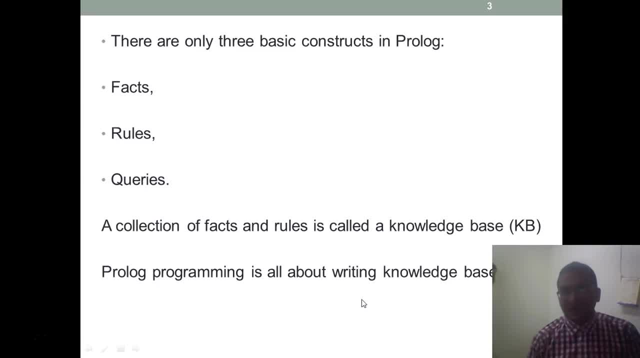 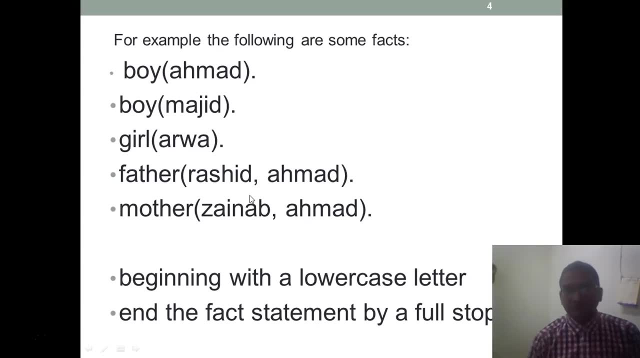 When we create a knowledge base for any agent, you can ask the queries. Let us take an example of some facts. That means we have given the fact that Ahmed is a boy, Mazid is a boy, Arwa is a girl, And then we have also given fact, like father, Rashid Ahmed. 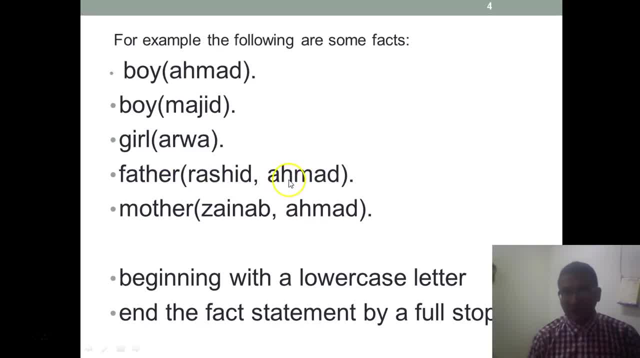 You can say Rashid is a father of Ahmed or Zainab is a mother of Ahmed. So in prologue terminology these Ahmed, Mazid and Arwa are said to be the atoms And boy girl is said to be the properties. 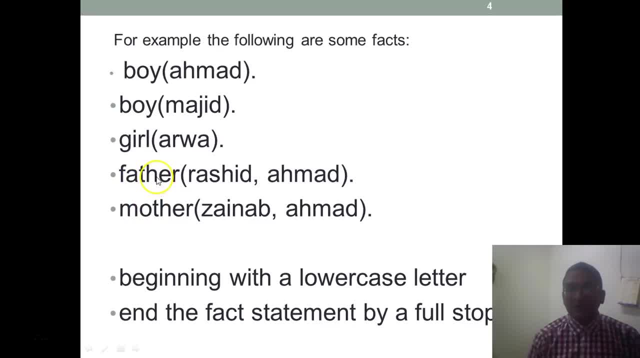 Whereas father and mother are the atoms, They are the relations. So when the properties are having two or more parameters, then it is said to be a relation. Now, while writing the facts in the prologue, we have to keep in mind certain rules. 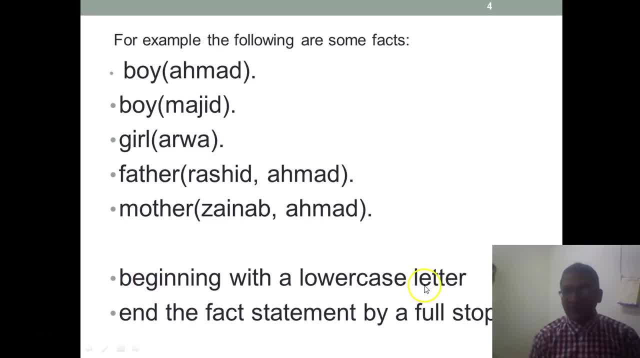 The first rule is beginning with a lower case letter. That is, always, when you write a fact, the first letter should be in lower case. The other important point that we have to keep in mind is that end the fact statement by a full stop. 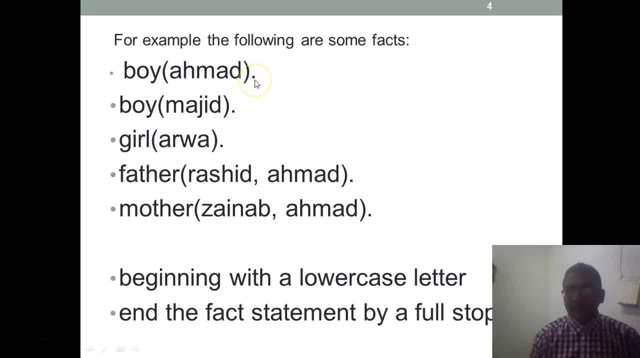 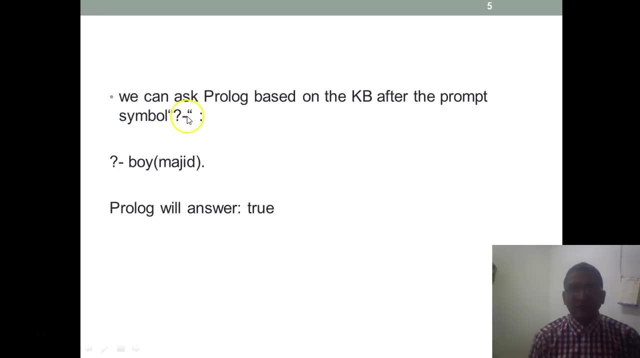 So every fact should be terminated by a full stop. So once you have created the knowledge base, then we can ask the query, like you can ask a prologue based on the knowledge base. after the prompt symbol, For example, if you ask a query. 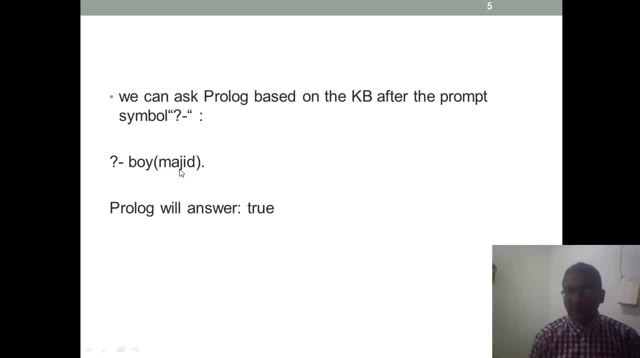 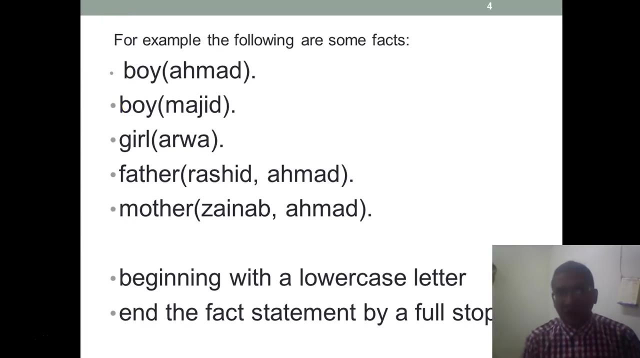 boy, Mazid. That means, is Mazid a boy? So, based on the given facts, you will get the answer true. So the answer for this is true. Similarly, if I ask, based on the given facts, is Rahima a girl? 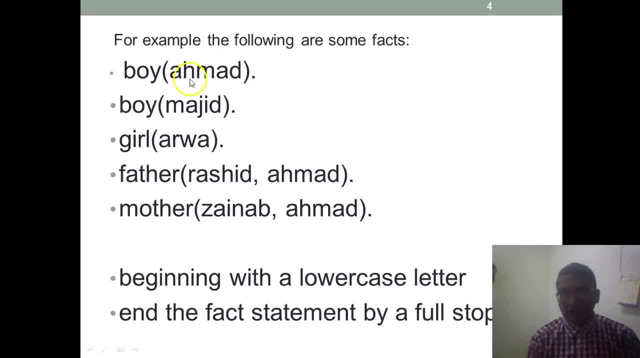 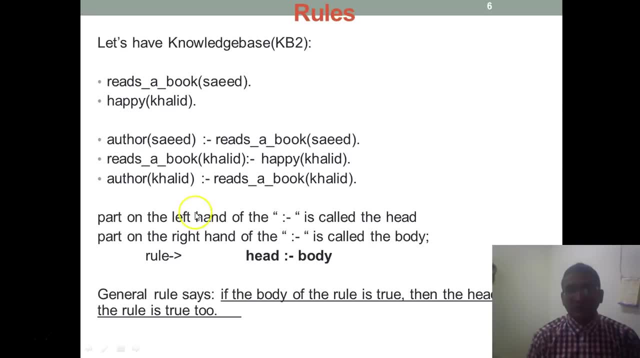 So if you look at this knowledge base, there is no information about Rahima, So the prologue will return the answer false. So now move on to the more wider knowledge base. So here we have facts and also we have the rule. Facts are a simple statement which contains only one atoms. 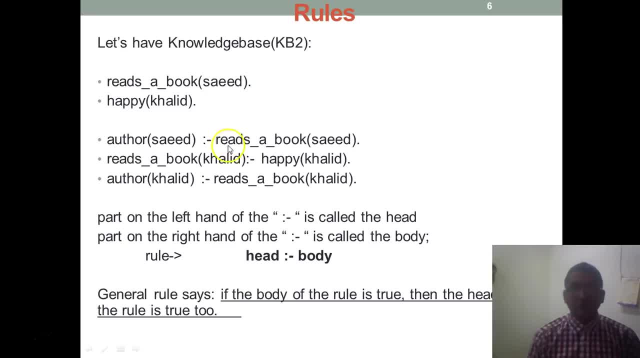 But when it comes to rule, rule is used to state the information which infers or implies, or implies to an other fact. So if we look at this knowledge base, we have read book Syed Happy Khalid. Then we have author Syed. 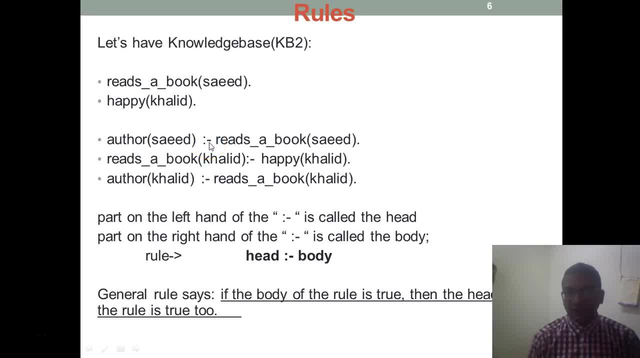 We are using the sign colon, followed by a hyphen sign. Read a book, Syed. So basically, when we talk of rule, we have two parts. One is the left hand side and one is the right hand side. The left hand side part is called the head of the rule. 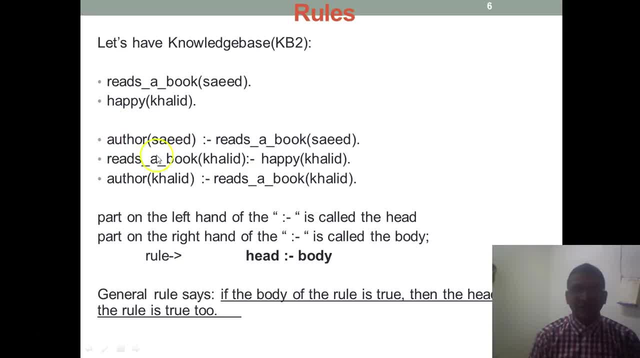 So if you look at this rule, this is the head and the right hand of this sign is called the body, So this part is called the body. The normal rule, or the general rule, says that if the body is true, then head is assumed to be true. 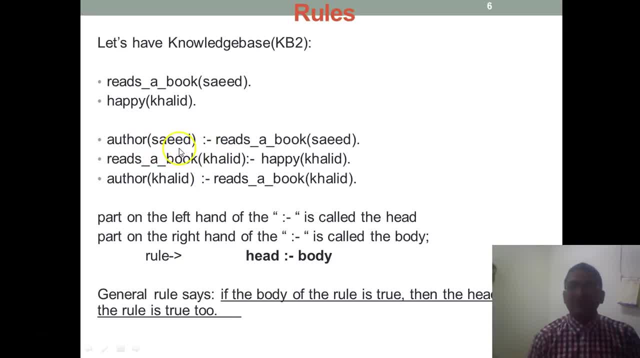 And how can you read this? We read this. Syed is the author. if Syed reads the book. Khalid reads the book if Khalid is happy. This is how we can represent the rules. Now let us look at some queries. that how we can frame a query. 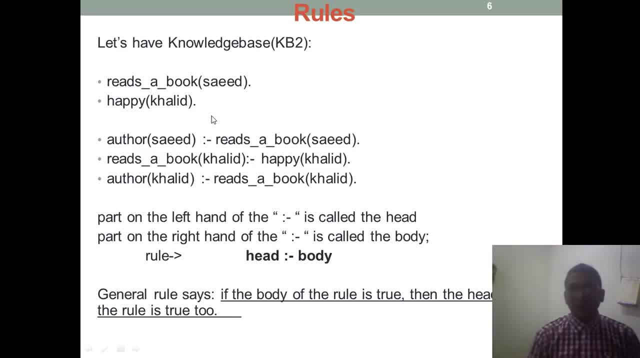 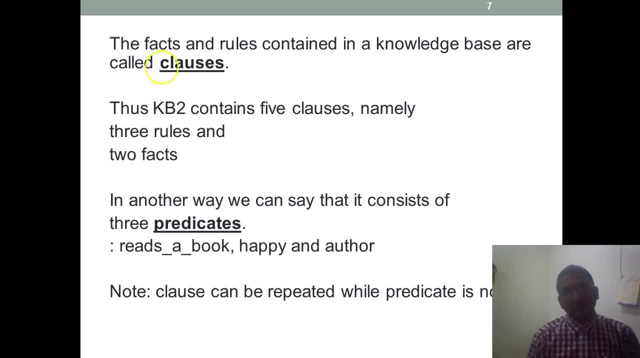 and how the answer should be written by the prologue. The fact and rules contained in the knowledge base are called clauses. So the collection of entire information which we are creating inside the knowledge base is basically a clauses. So in the knowledge base, basically we have the facts and the rules. 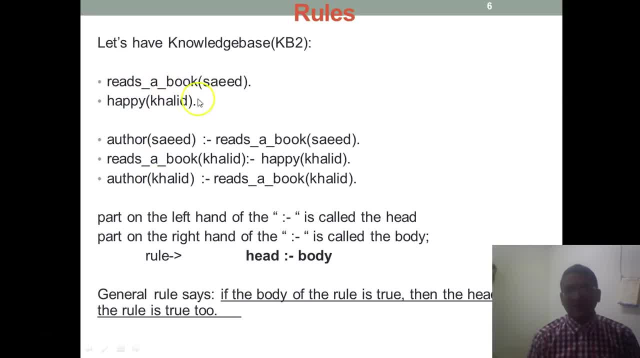 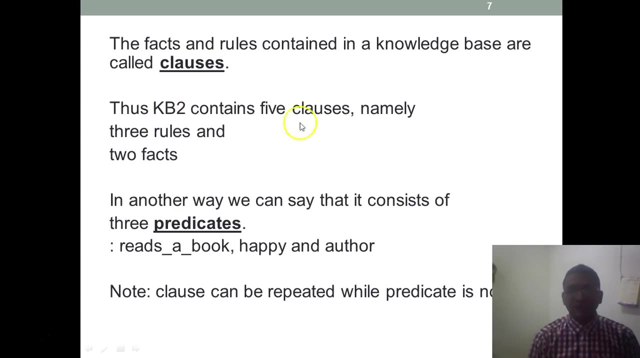 So all the facts and rules are collectively called as clauses. So if we look at this knowledge base, it contains five clauses, out of which two are the facts and three are the rules. The another way we can say that it consists of three predicates. 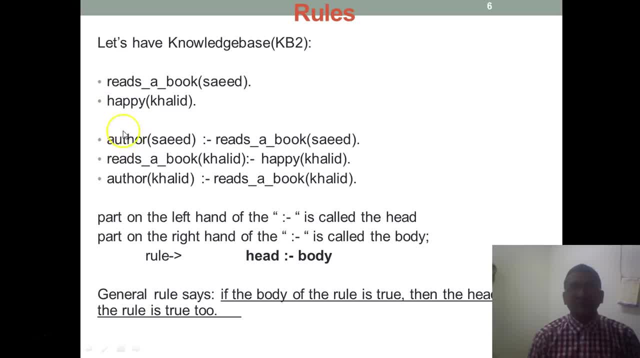 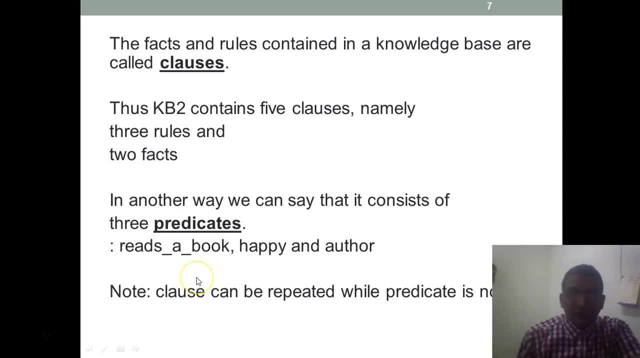 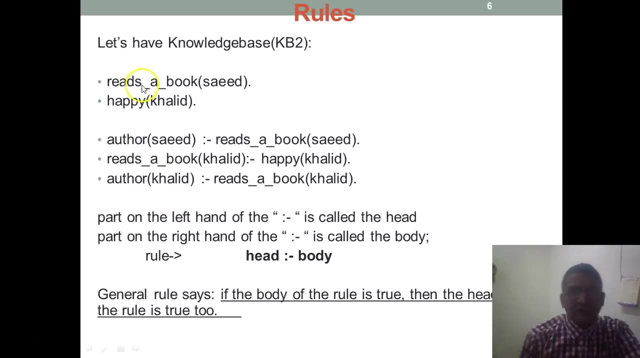 Predicate means. so predicates are a unique set of information that we have created in the knowledge base. So if you look at this, in this knowledge base we have five clauses Out of five clauses. we are saying these are two facts and the three are rules. 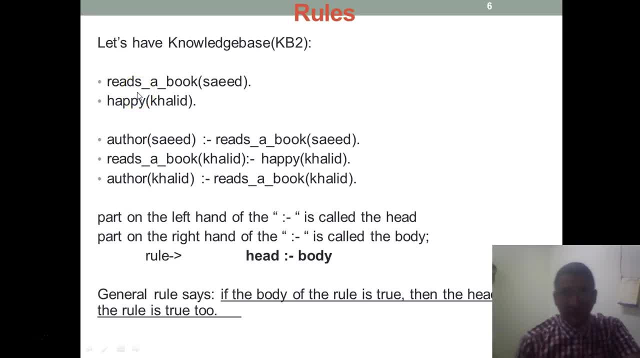 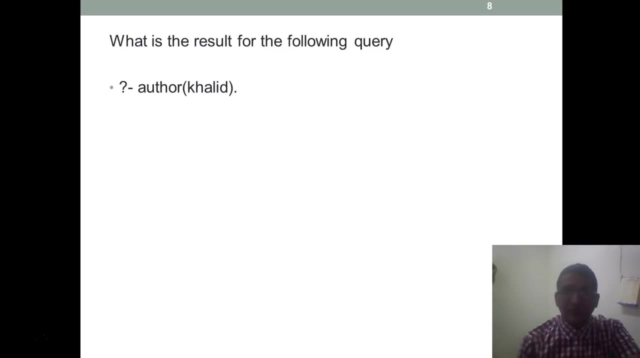 But if we say that the unique information we can see, we have three unique facts. One is read a book, happy and about the author, So we have. we can also say that this knowledge base contains three predicates. So now we look at the query. 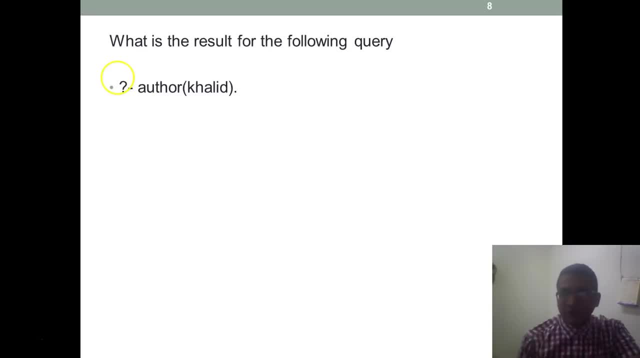 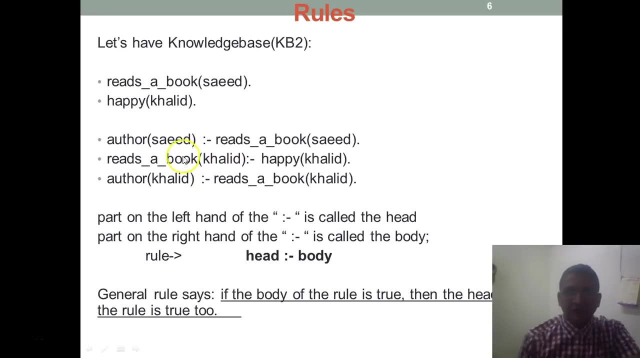 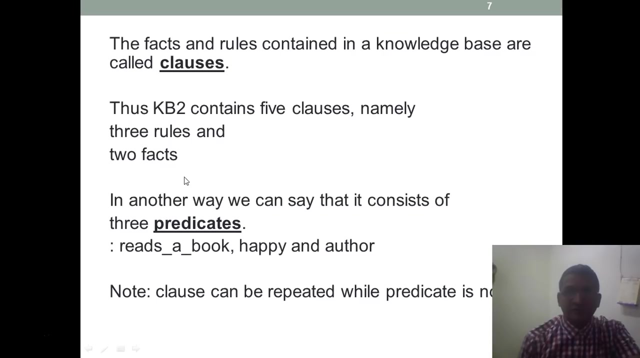 Khalid author means you want to ask to the prologue. that is Khalid an author? So if you look at this knowledge base, we don't have the information Khalid author. So what does it return? It will return true, True.